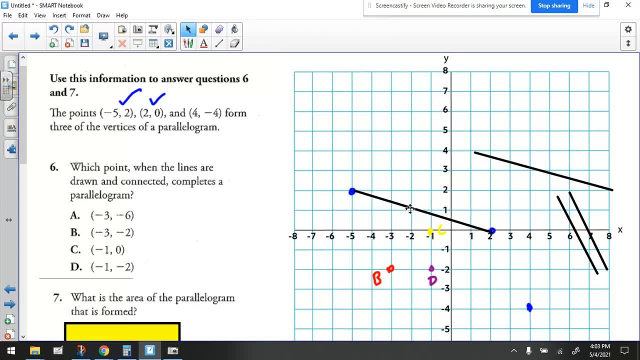 to remind you about This line right here. that has to be one of the lines to the parallelogram. I didn't draw that quite perfect. Maybe we should straighten that just a little touch Now. that means that the opposite would have to be the same length. the opposite side. 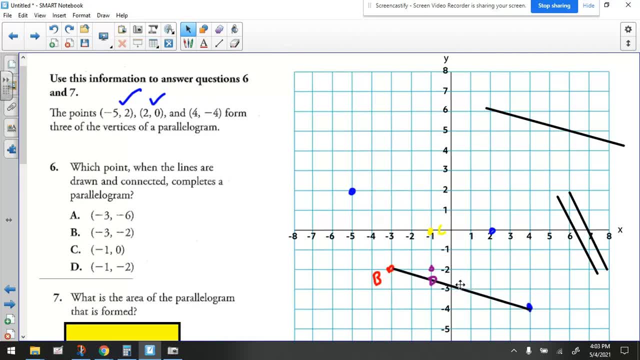 So if I take the opposite side and I draw the opposite side, I'm going to draw the opposite side. So if I take the opposite side and I draw the opposite side, I'm going to draw the opposite side. Maybe we should take the same line and move it over, right? 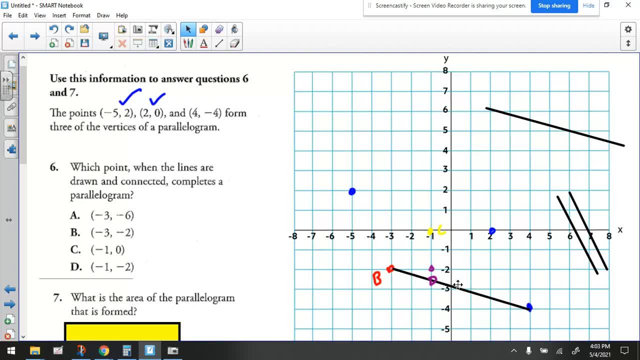 See. look at the answer choice B. The answer choice B is negative 3, negative 2.. So so far it's lining up with answer choice B. Now keep in mind that in fact let me clone this and move it over here. 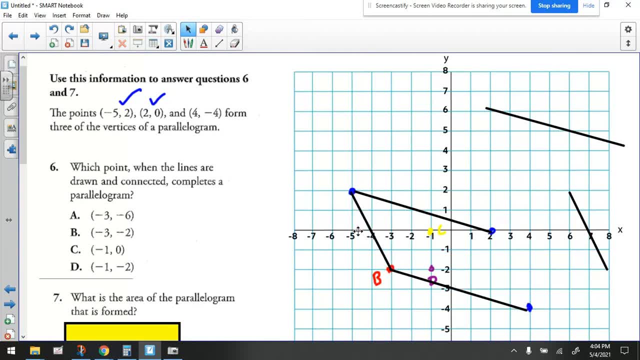 Keep in mind that, also going this way, these have to be equal in parallel. So whatever the distance is between these two dots, it has to be the same for these two. They have to be parallel. So let me just move this, Let me delete that. 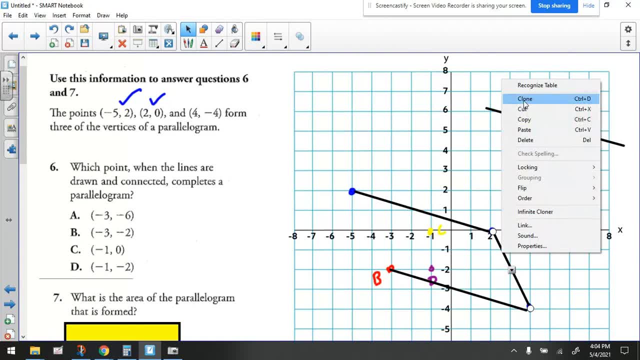 And if I clone this, it'll be at the same angle. Clone that. So there's a clone. See it's the same thing. And if I slide it over, see that means that choice B is looking pretty good Where choice C, D and A. you know, there's no way that's going to work. 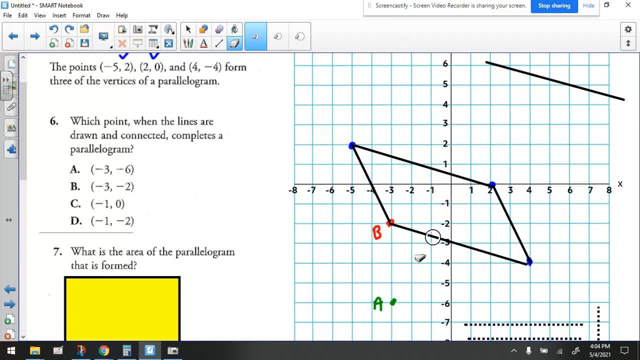 So let me just go ahead and erase those other choices, And I'm hoping that you can now see that it's definitely going to be choice B that'll form the parallelogram, Because, remember, for it to be a parallelogram, the opposite sides have to be parallel and they have to be congruent. 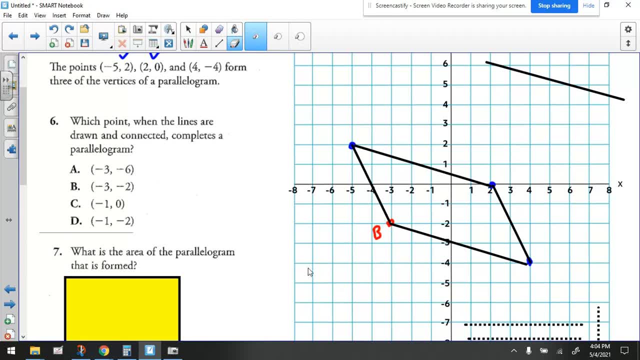 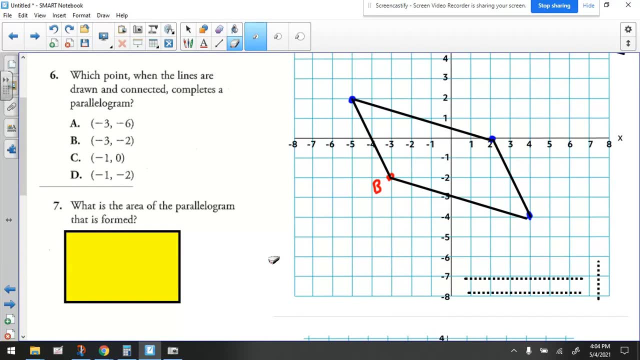 And that's really the only spot where we can get that to be true. All right, so the second part, number seven, says what is the area of the parallelogram formed And the issue that we have here. none of the lines match up with the blue. 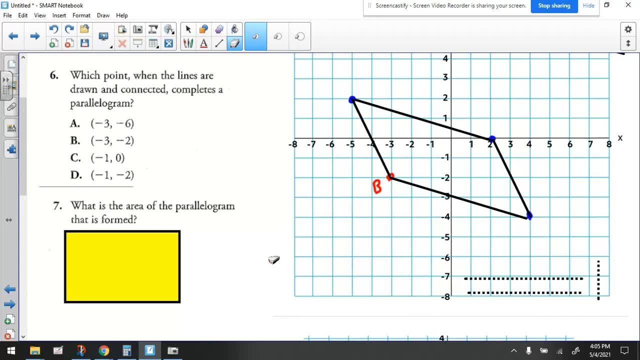 Grid lines that you see for the coordinate plane. So when that's true, then you have to decompose the figure into shapes that do fall on the lines for the coordinate plane, And that may be difficult for you to see that. So I'm just going to use this little dotted line to help you. 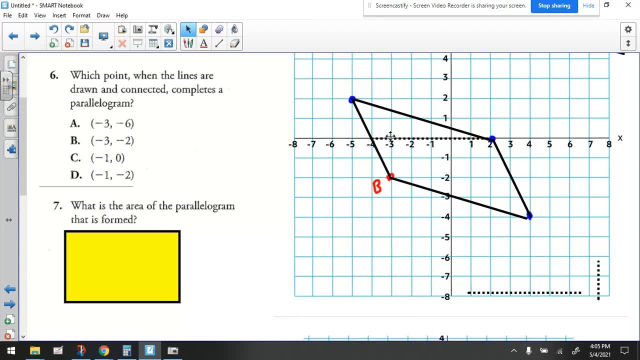 If we look see how here we can find the area of this top triangle that's formed, And if I do that again down here, do you see how we have this triangle down here that we could find the area of, Because we would have the base. 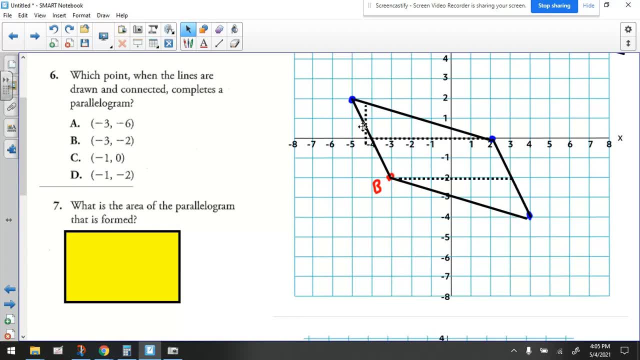 And we would have the height of that triangle. And likewise, here we would have the base and we would have the height of this triangle. And if you look in the center you can see that we end up having another parallelogram. So I'm going to use different colors to highlight, just so that you can see what shapes I'm talking about. 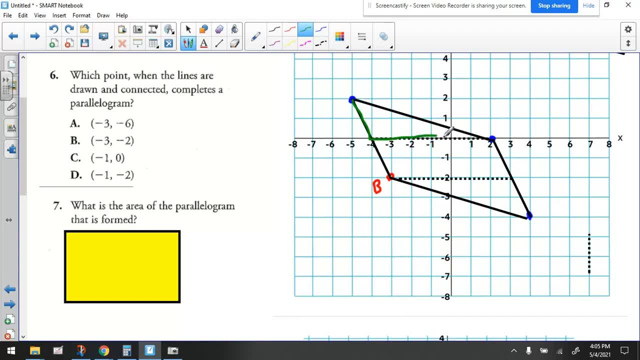 We're going to find the area of- I'm going to trace this in green. We're going to find the area of this green triangle And I apologize if that's not perfect. We're going to find the area of this red parallelogram. 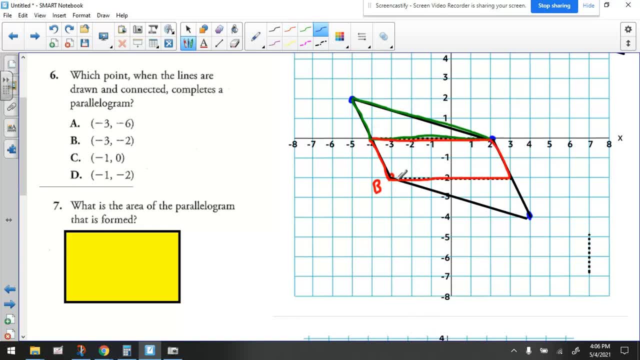 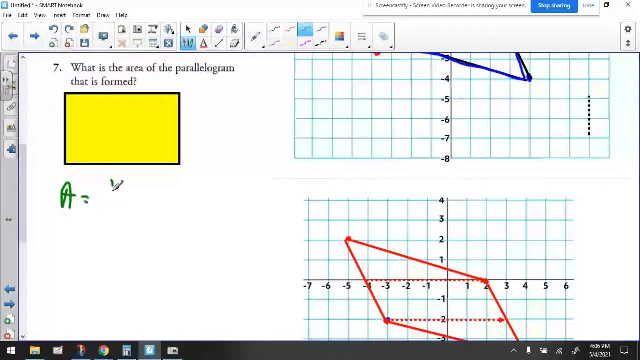 And we're going to find the area of this blue triangle on the bottom, Because all that lines up with the grid lines. So let's start with the green triangle. The formula for area of a triangle is: area equals half of the base times the height. 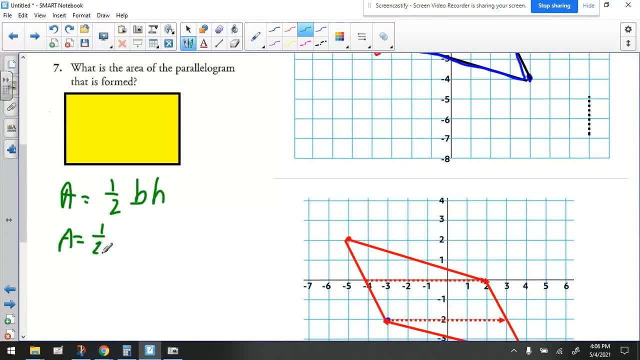 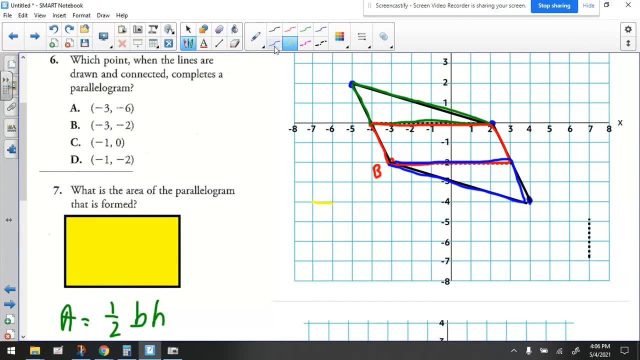 Area equals half. Now we have to figure out what the base is. So we're going to use this dotted line to represent the base And remember this line right there. that's one unit, So if we count, I'm just going to move this over. 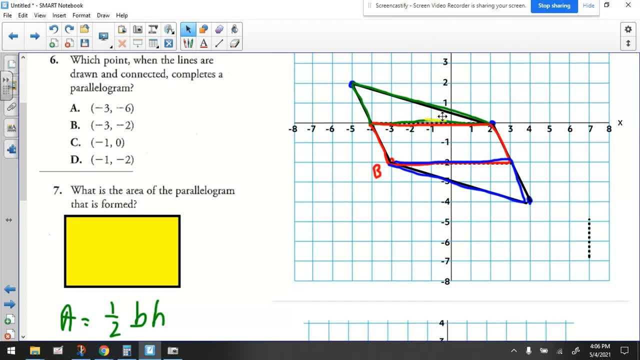 If we count, see, that's one, two, three, four, five, six, Six units And by the way, it looks like the blue one also will be six: One, two, three, four, five, six. So the basis for both of those triangles we can use six. 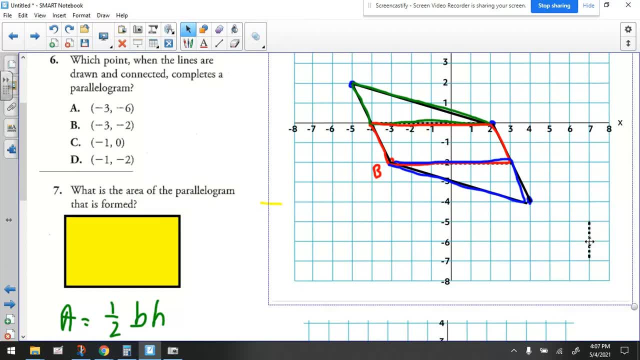 Now, if we use this little dotted line here, Let me move this dotted line over here To show you. Now, remember, the height has to be perpendicular to the base And we can have that be anywhere along that dotted line that I have underneath it. 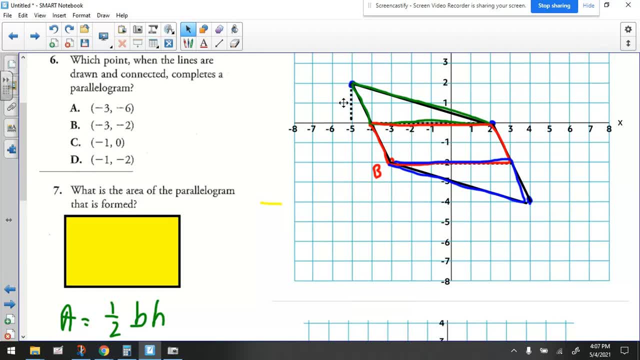 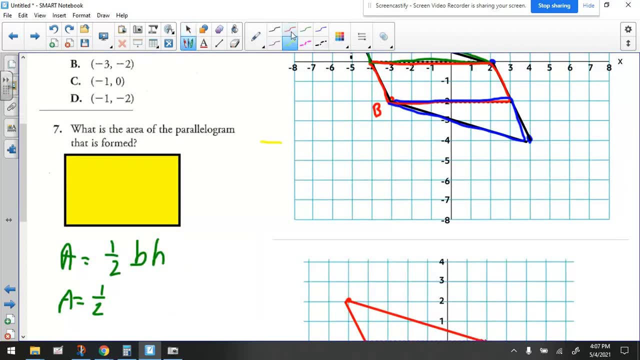 But usually we look at that opposite vertex And if you look at the length of this dotted line, you can see that that's two units, All right. So we have a base of six And we have a height of two, All right. 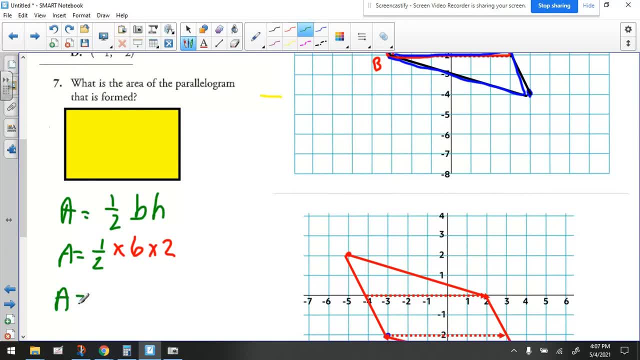 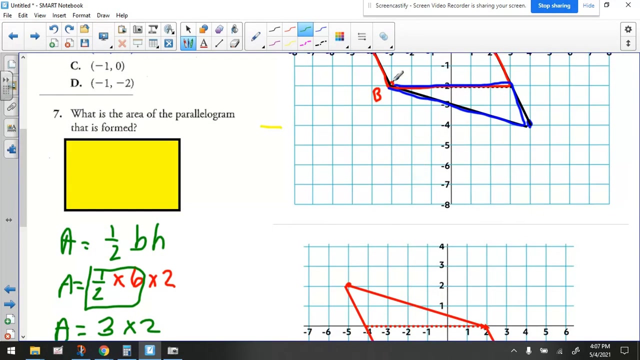 Next, We can go Go ahead and take half of six, which would be three, And multiply that times two, which would end up being six square units. That's a six. Sorry about the mess there, All right. And if we look at the blue triangle, we already counted that the base on here is six. 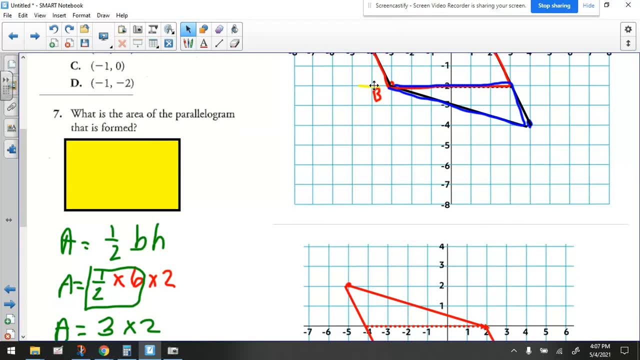 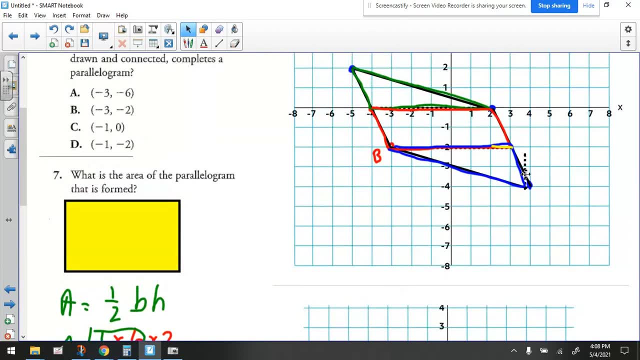 This is six units, So let me just show you that again in case you're confused: One, two, three, Four, five, six And the height on that if we go parallel, I'm sorry, perpendicular is what I meant to say. 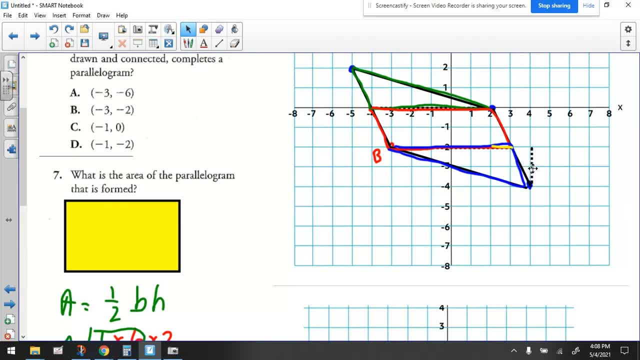 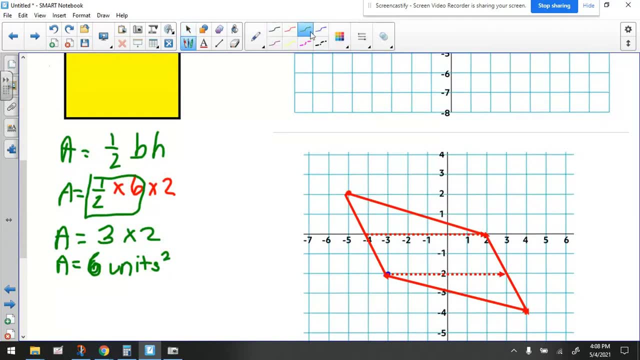 With the base on that and we go all the way to this opposite vertex. you can see that that also has a height of two. So really we're doing the same exact thing to get the area of the blue triangle And we can go through the process of writing all this stuff down again. 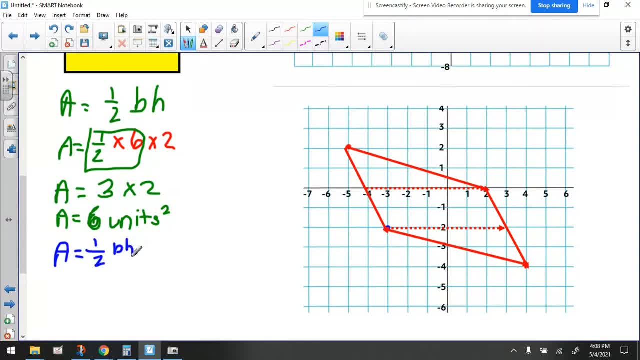 But it's really the same formula and the same dimensions, Right? So we're looking at half of six. All right, So we're looking at half of six. All right, So we're looking at half of six. Six times two, we're going to get the same thing. we just got above, right? 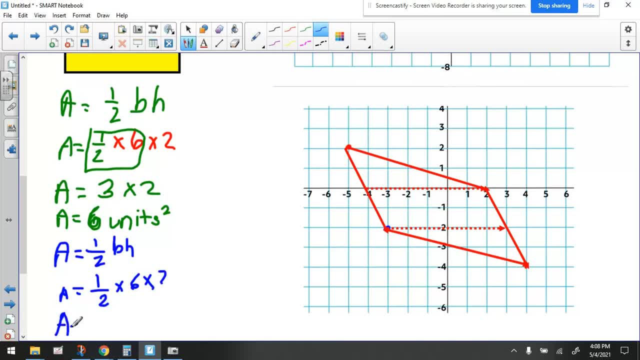 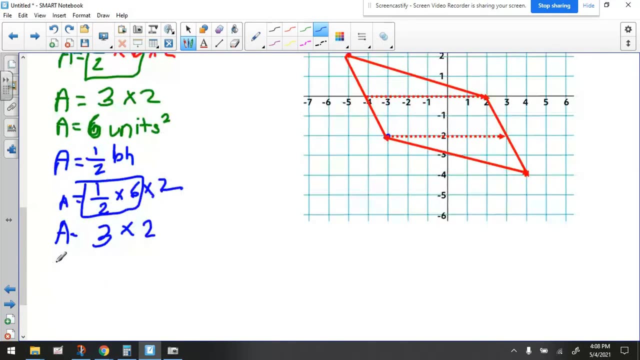 We would still do. well, my mouse is getting a little difficult to write neatly with for some reason. Maybe it's my hands getting tired. So if we take half of six, you know we're still going to get that three. And if we do three- by the way this is a two times two- we're still going to get six. 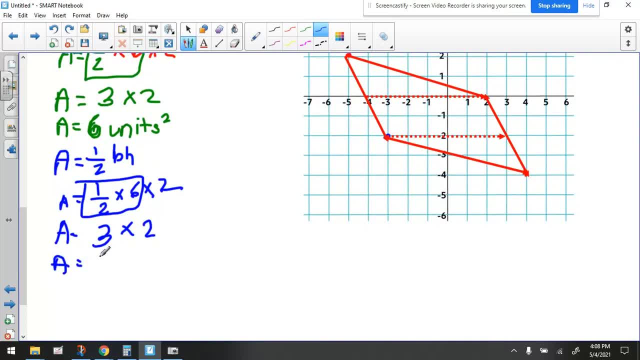 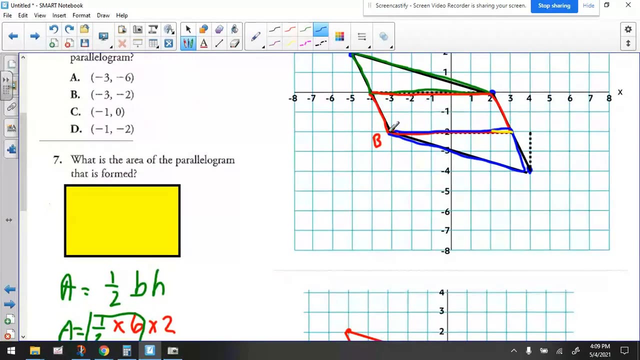 So the blue triangle has an area of six square units. All right, Now what about the parallelogram in the center? Let's take a look at that And I'll highlight it again in red. Here it is in red Now. we already counted here, right? 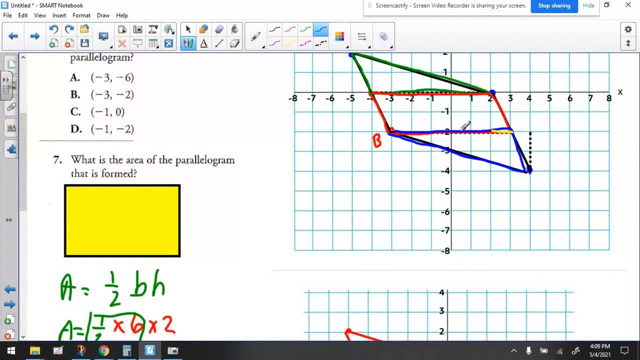 One. We already know that this is six and we can use that as the base. And if we look at the height of this thing- remember the height has to be perpendicular to the bases And you see that that has a height of two.